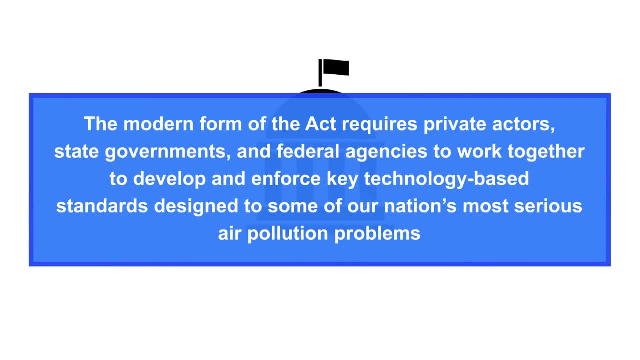 the Clean Air Act several times since it was passed. The modern form of the act requires private actors, state governments and federal agencies to work together to develop and enforce key technology-based standards designed to some of our nation's most serious air pollution problems. 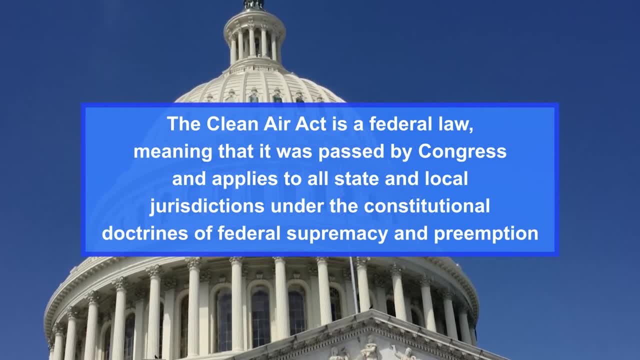 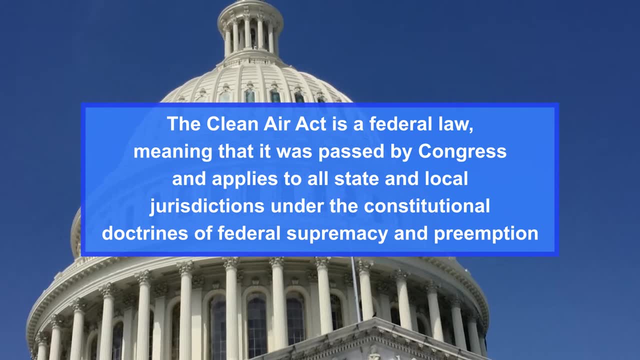 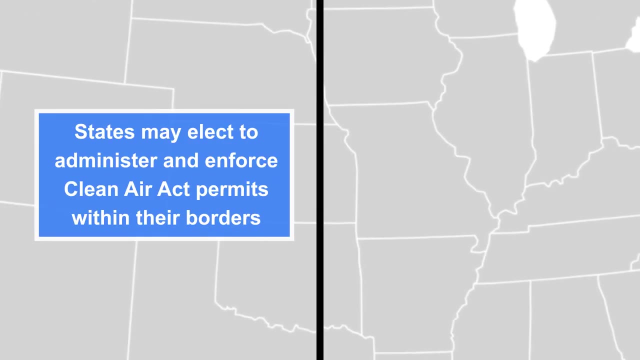 The Clean Air Act is a federal law, meaning that it was passed by Congress and applies to all state and local jurisdictions under the constitutional doctrines of federal supremacy and preemption. However, state governments have some latitude in the administration of the law. For example, states may elect to administer and enforce Clean Air Act permits within their borders. 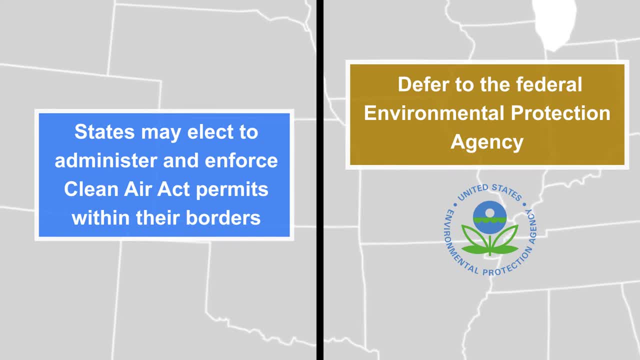 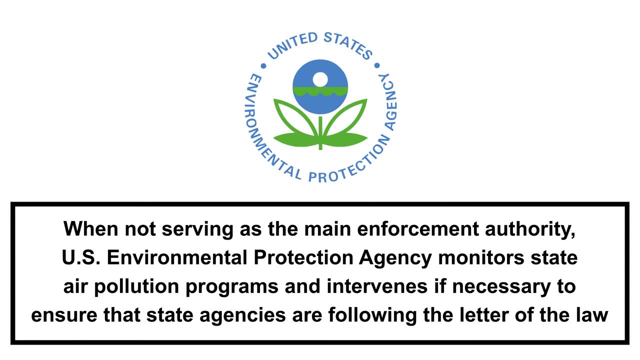 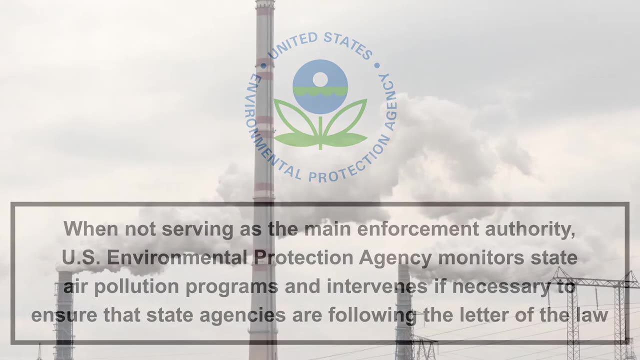 or they may defer to the Federal Environmental Protection Agency When not serving as the main enforcement authority. US Environmental Protection Agency monitors state air pollution programs and intervenes if necessary to ensure the state agencies are following the letter of the law. Some states have gone so far as to. 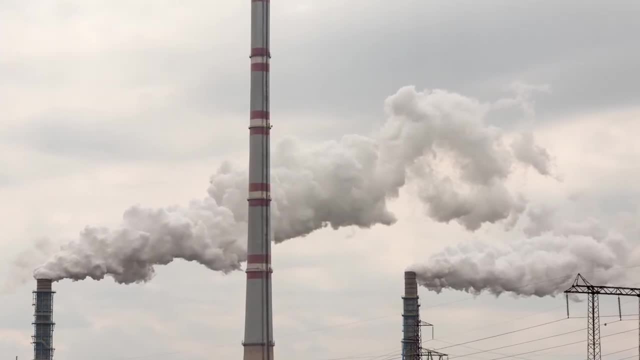 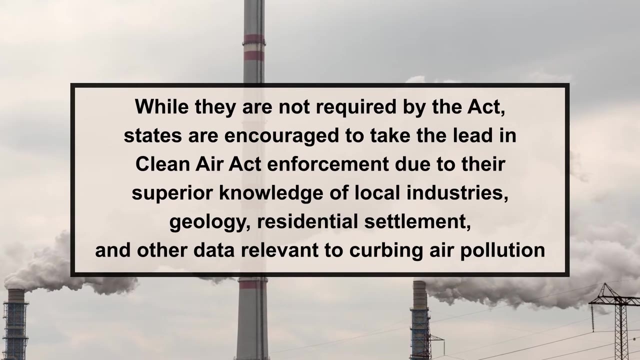 create their own, more stringent air pollution protection programs, as the Clean Air Act sets only the mandatory minimum standards. While they are not required by the act, states are encouraged to take the lead in Clean Air Act enforcement due to their superior knowledge of local industries. 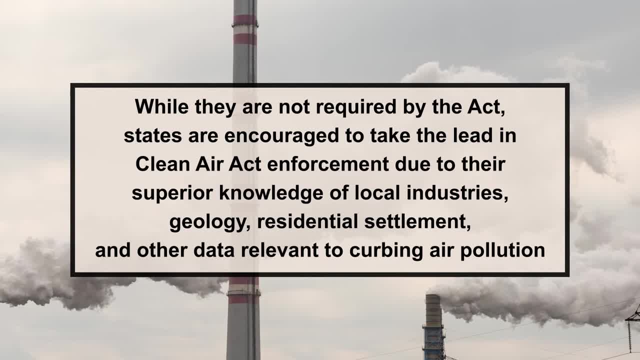 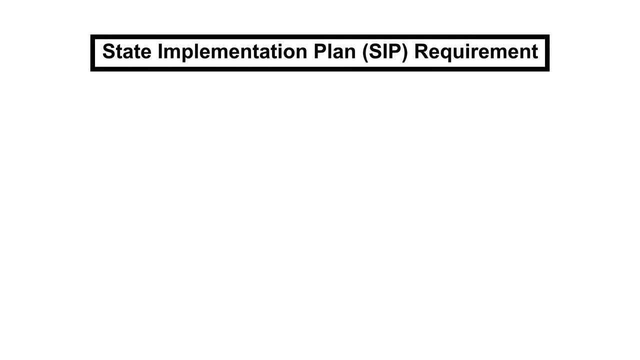 geology, residential settlement and other data relevant to curbing air pollution. The State Implementation Plan SIP requirement is one aspect of the Clean Air Act, under which state governments have very little or no control over the state's air pollution. The Act requires the EPA to set specific standards for six common pollutants. 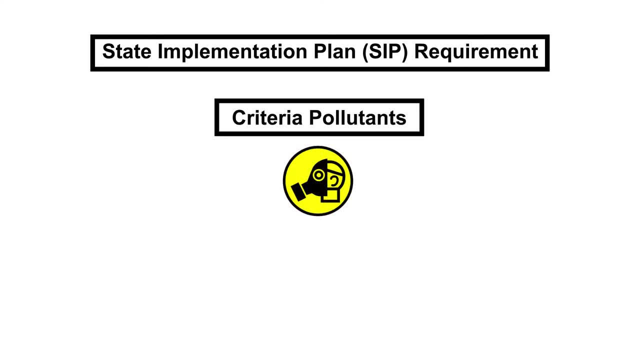 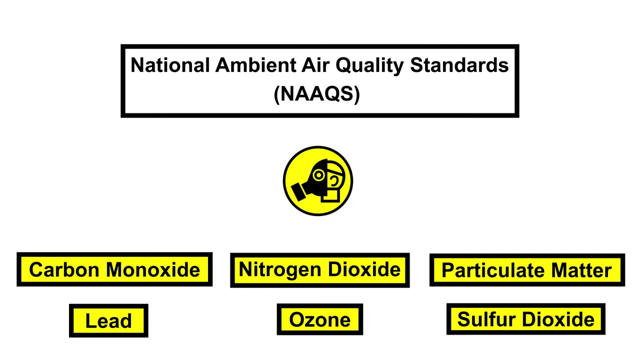 known as the criteria pollutants proven to damage property and harm human health in the environment – carbon monoxide, lead, nitrogen dioxide, ozone, particulate matter and sulfur dioxide. These limits known as the National Ambient Air Quality Standards, or NACs. 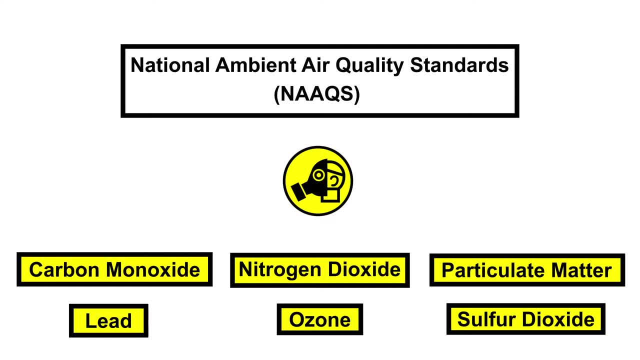 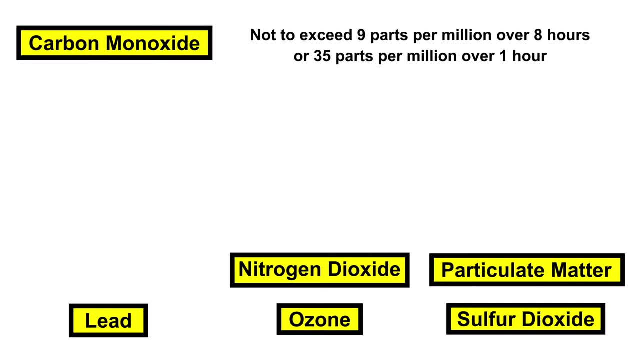 create headline standards for the six criteria pollutants. carbon monoxide may not exceed 9 parts per million over 8 hours or 35 parts per million over 1 hour. Lead is limited to 0.15 micrograms per cubic meter. Nitrogen dioxide can be only 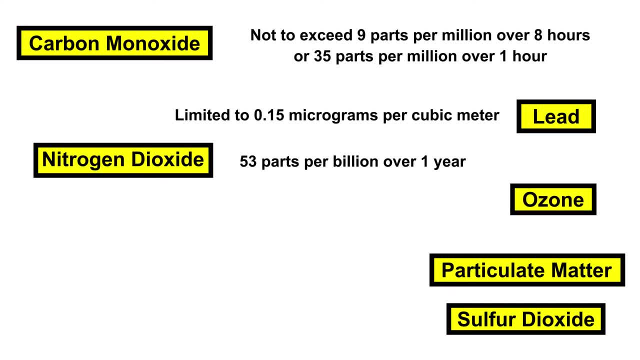 53 parts per billion over 1 year. Ozone must 0.07 parts per million or less over 8 hours, Particulate matter can be no more than 35 micrograms per cubic meter over 24 hours And sulfur dioxide can be no more than 35 micrograms per cubic meter over 24 hours. 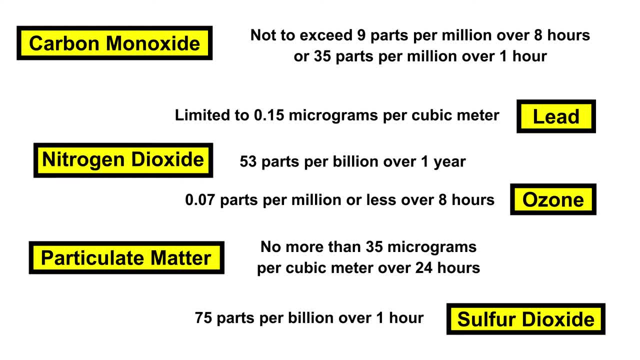 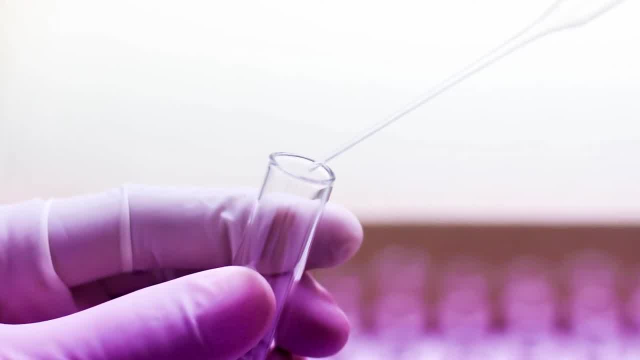 And sulfur dioxide limits are set at 75 parts per billion over 1 hour. The EPA sets the NACs using the best information available at the time and revises the standards as necessary Once the NACs are in place, the Clean Air Act requires. 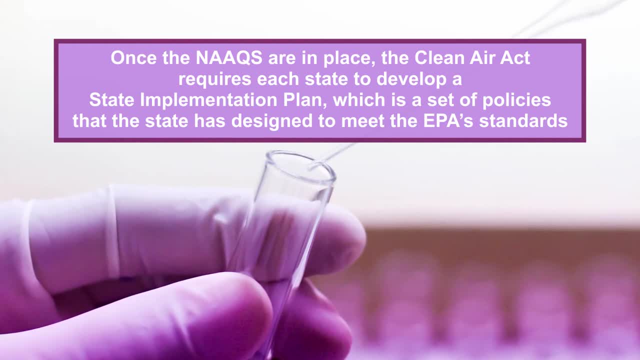 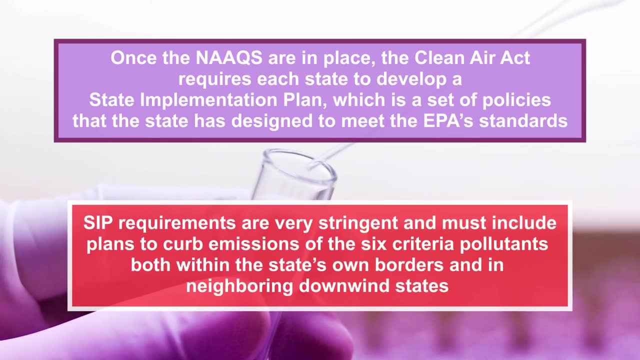 each state to develop a state implementation plan, which is a set of policies that the state has designed to meet the EPA's standards. SIP requirements are very stringent and must include plans to curb emissions of the six criteria pollutants. The NACs must include plans to curb emissions of the six criteria pollutants, both within the state's 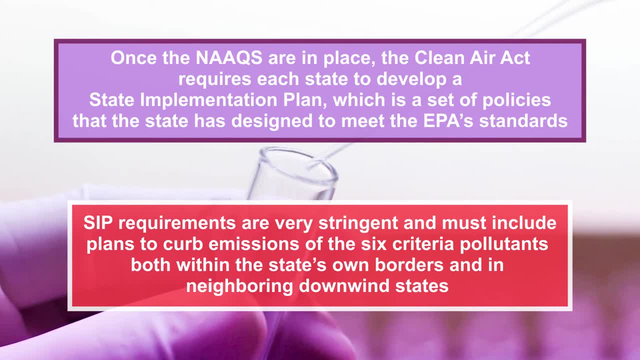 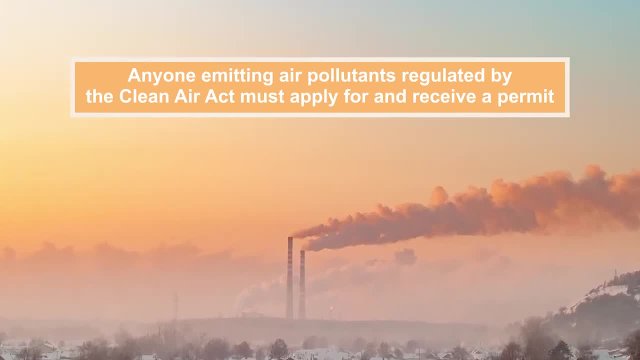 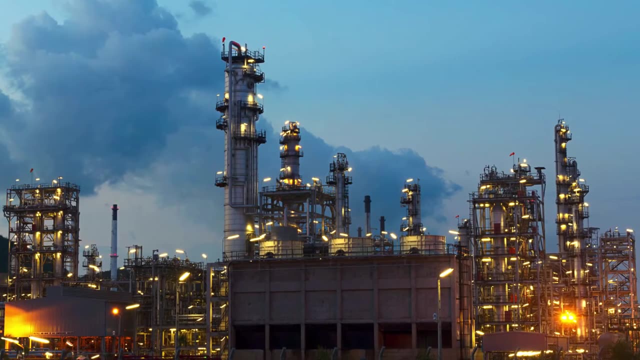 own borders and in neighboring downwind states. Regardless of type or source, anyone emitting air pollutants regulated by the Clean Air Act must apply for, and receive, a permit. Standards for award of a permit vary based upon the type of pollutant and the type of source emitting the. 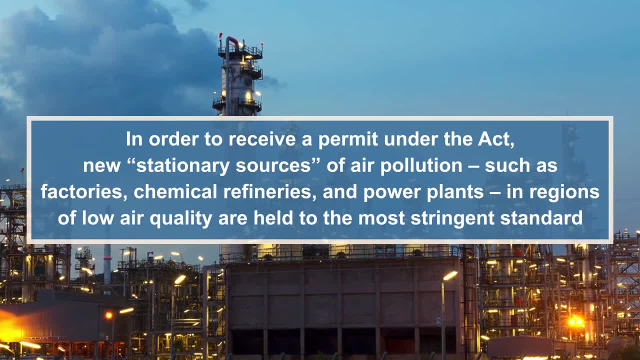 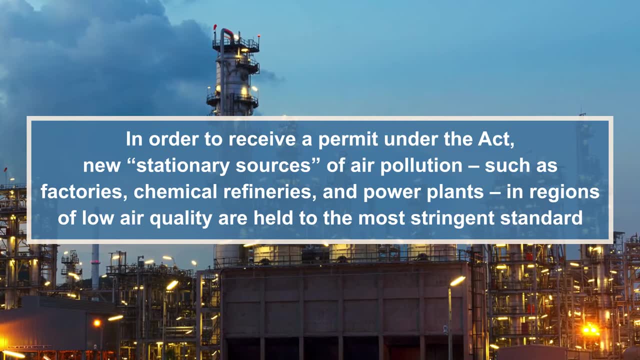 pollutant. In order to receive a permit under the Act, new stationary sources of air pollution, such as factories, chemical refineries and power plants, must be provided. The NACs must also include plans to curb emissions of the six criteria pollutants. 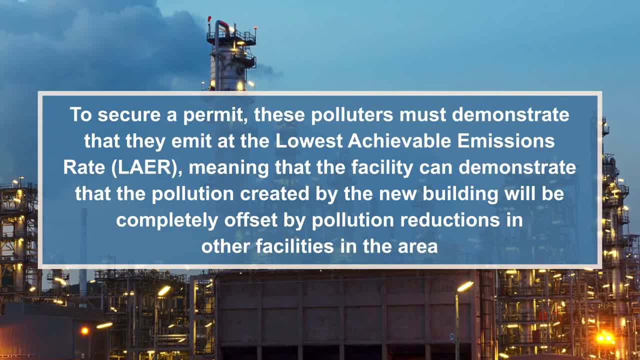 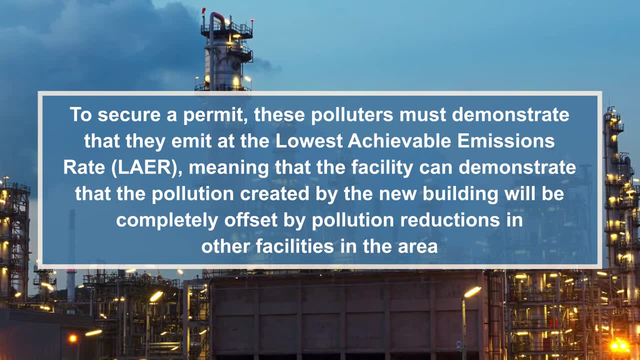 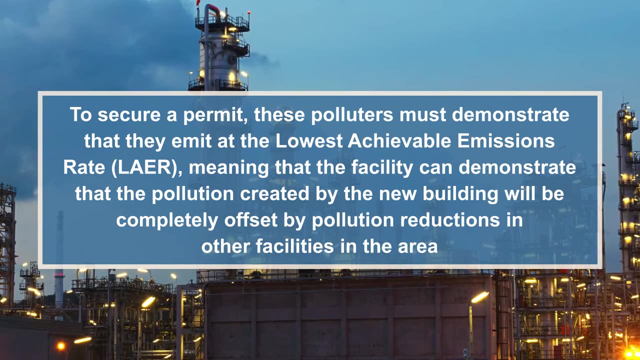 To secure a permit, these pollutants must demonstrate that they emit at the lowest achievable emissions rate, LAER, meaning that the facility can demonstrate that the pollution created by the new building will be completely offset by pollution reductions in other facilities in the area. This requirement can add substantial cost to a proposed project and is designed to 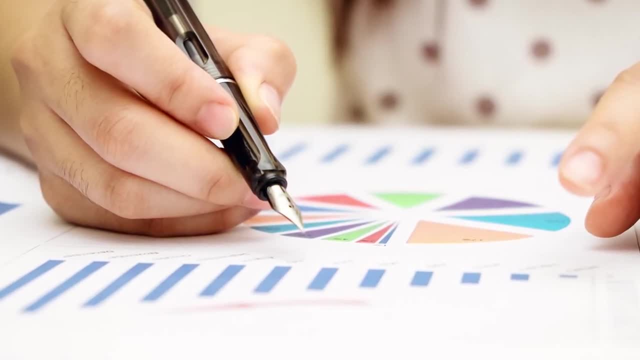 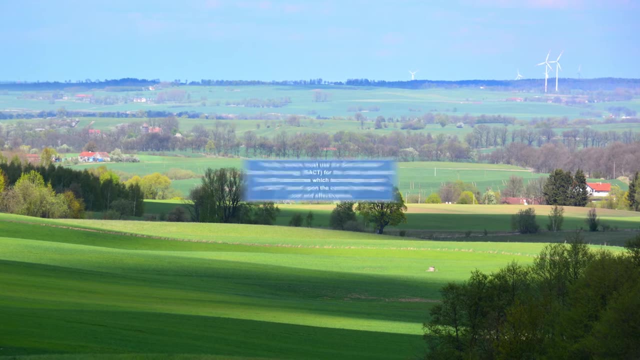 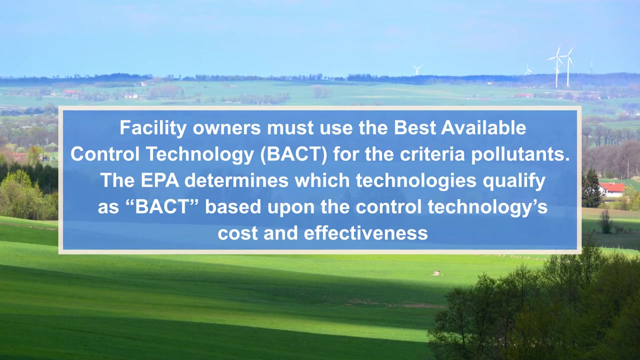 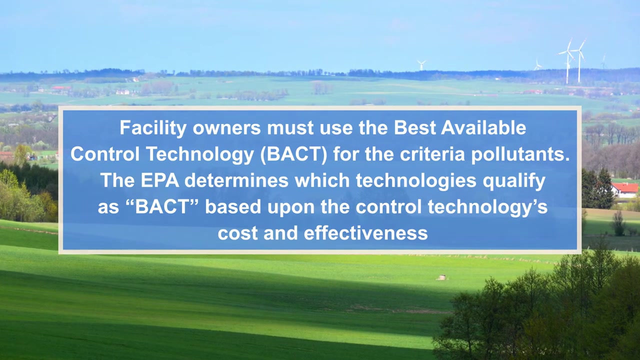 deter development of polluting industries in areas already in the area For new or substantially modified sources of air pollution. in areas with good air quality, facility owners must use the best available control technology for the criteria pollutants. The EPA determines which technologies qualify as BA-CT based upon the control technology's cost and effectiveness. Once the EPA has identified a certain technology as meeting the BA-CT standard, it becomes mandatory for all new sources of air pollution. 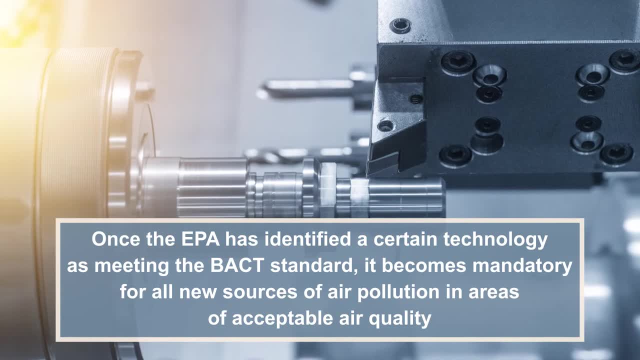 It makes it possible to control air pollution by using theこちら criteria, and it is needed in the area of energy efficiency. The EPA must also clarify any technology requirements for the net quality of air pollution. sources of air pollution in areas of acceptable air quality. 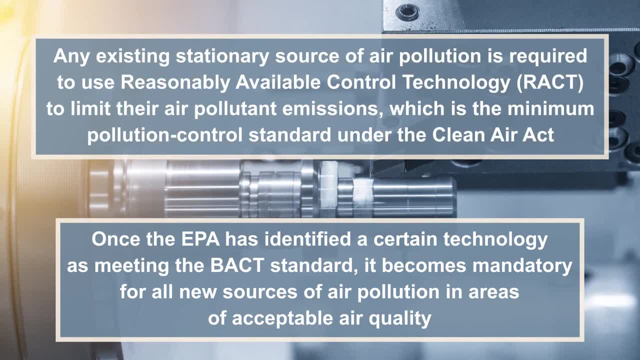 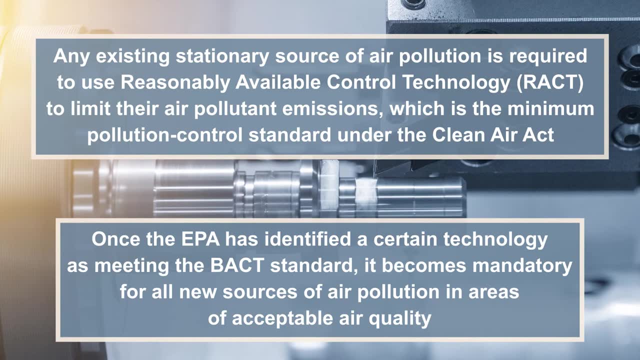 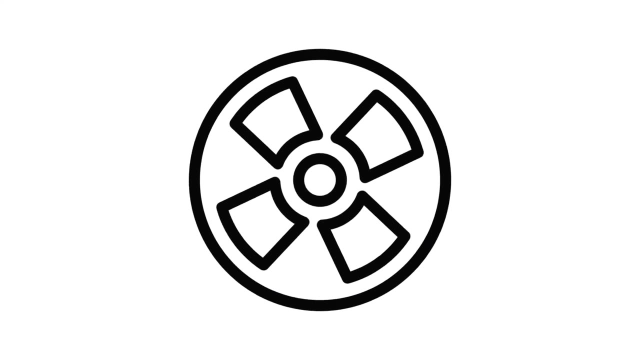 Any existing stationary source of air pollution is required to use Reasonably Available Control Technology to limit their air pollutant emissions, which is the minimum pollution control standard under the Clean Air Act. The Clean Air Act regulates many contaminants beyond the six criteria pollutants under the. 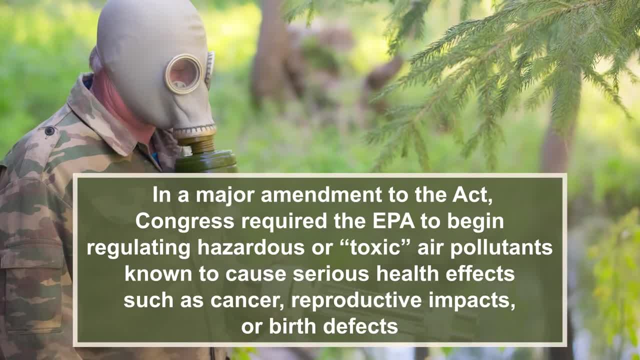 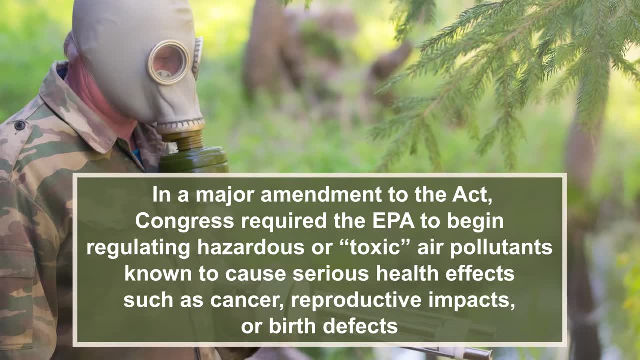 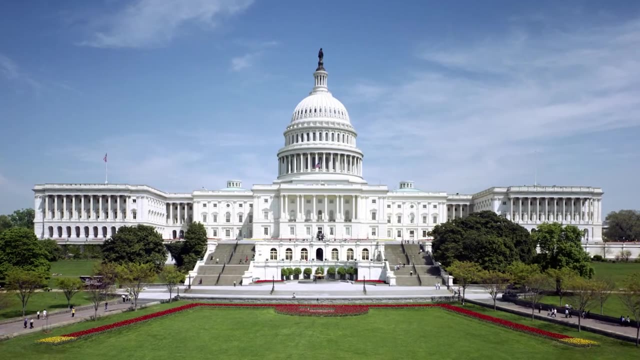 NAICS program. In a major amendment to the Act, Congress required the EPA to begin regulating hazardous or toxic air pollutants known to cause serious health effects such as cancer, reproductive impacts or birth defects. Congress took a very strong position with the new national emission standards of hazardous 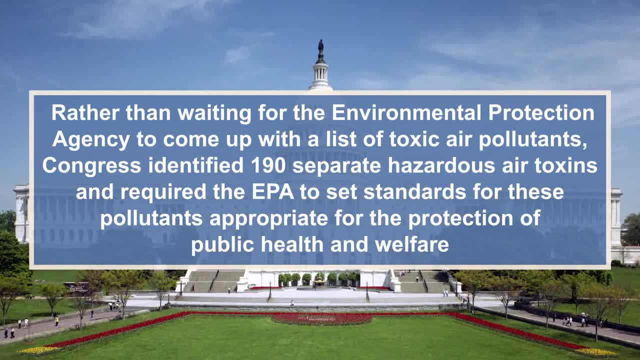 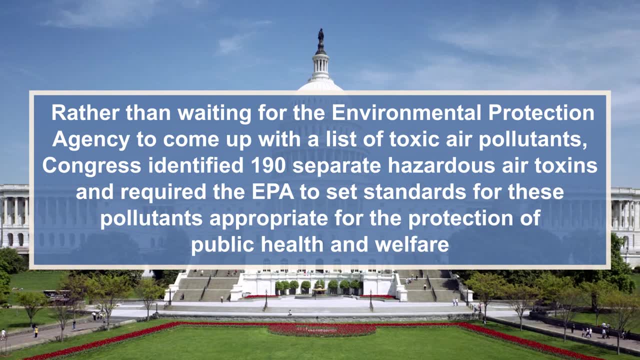 air pollutants, Rather than waiting for the Environmental Protection Agency to come up with a list of toxic air pollutants, Congress identified 190 separate hazardous air toxins and required the EPA to set standards for these pollutants appropriate for the protection of public health and welfare. 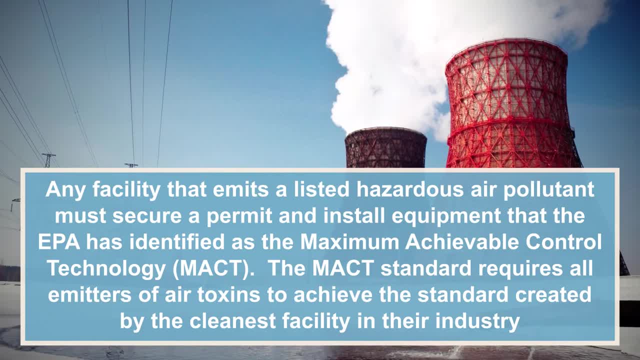 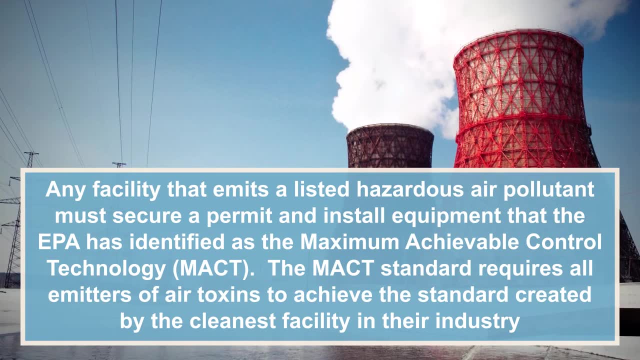 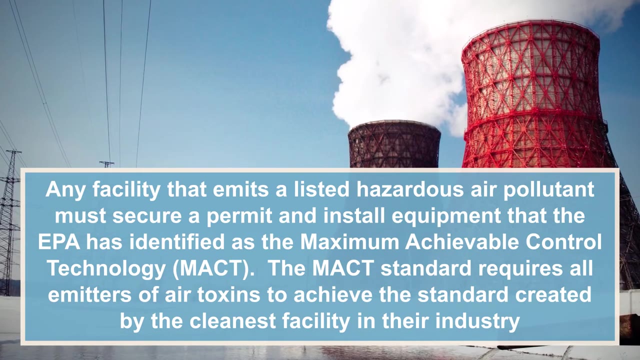 Any facility that emits a listed hazardous air pollutant must secure a permit and install equipment that the EPA has identified as the Maximum Achievable Control Technology. The MA-CT standard requires all emitters of air toxins to achieve the standard created by the cleanest facility in their industry. 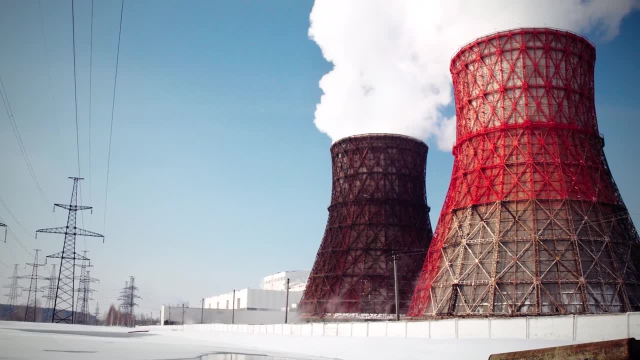 In other words, the MA-CT benchmark shifts as emissions control technologies continue to develop, But all similar facilities are held to the standard of their highest quality. The MA-CT benchmark is still in development. The MA-CT standard is still in development. 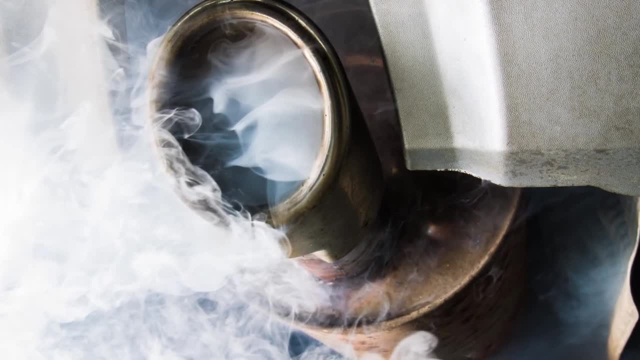 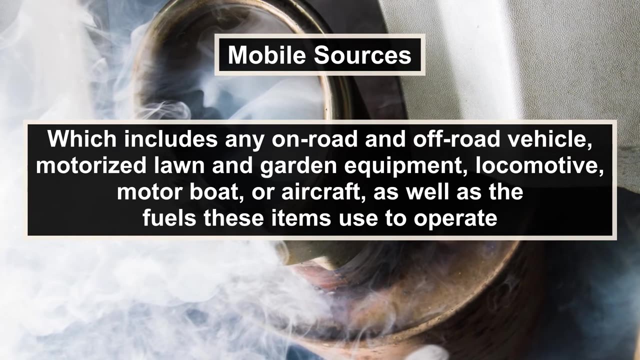 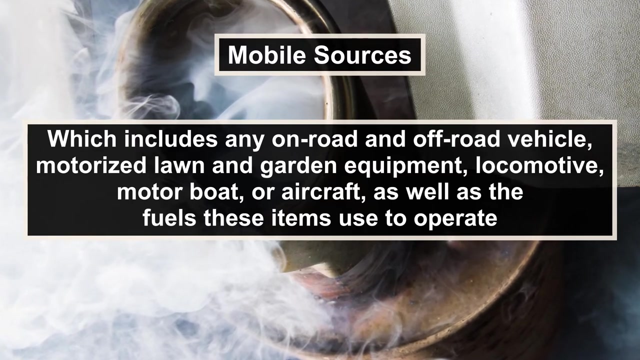 achieving competitor. Congress has also directed the EPA to issue standards for mobile sources, which includes any on-road and off-road vehicle, motorized lawn and garden equipment, locomotive, motorboat or aircraft, as well as the fuels these items use to operate. The EPA enforces: 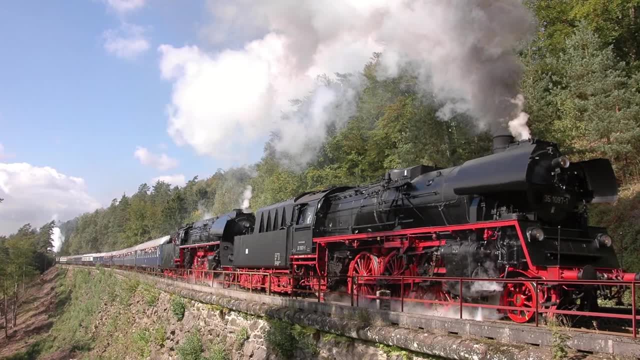 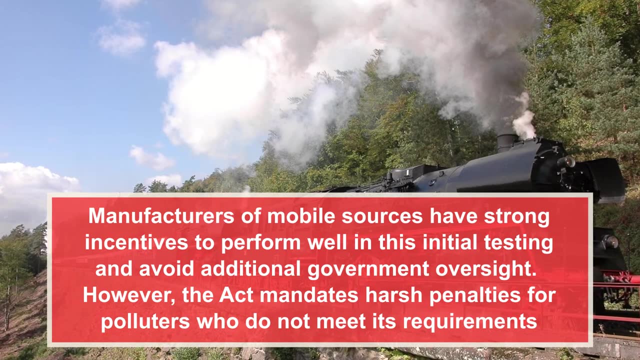 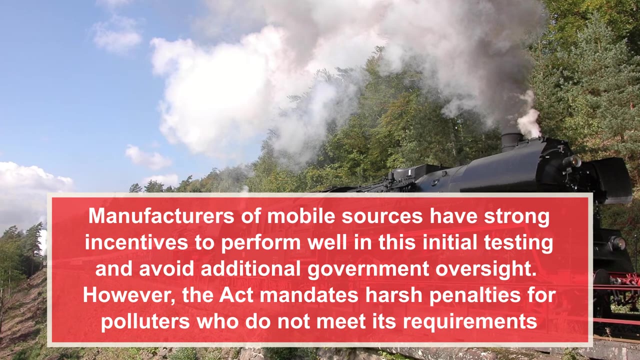 its mobile source standards through mandatory testing and certification of new technologies. Manufacturers of mobile sources have strong incentives to perform well in this initial testing and avoid additional government oversight. However, the Act mandates harsh penalties for polluters who do not meet its requirements, Knowing an intentional violation. 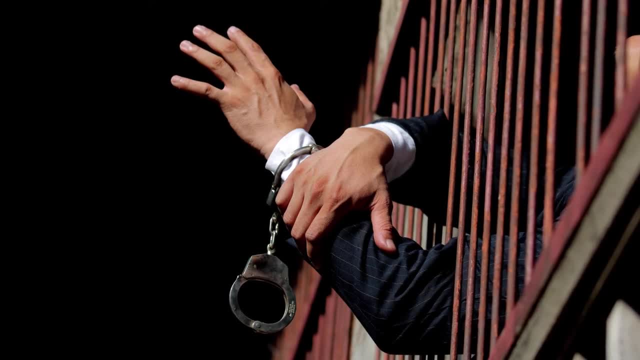 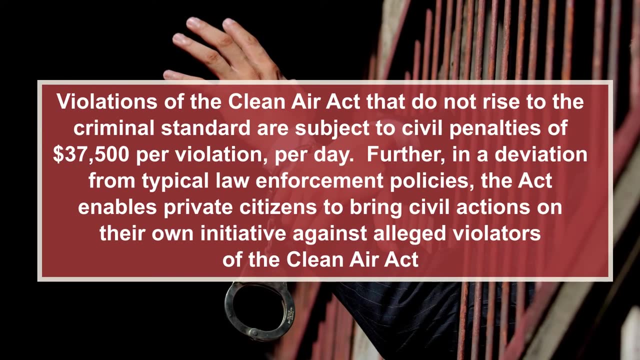 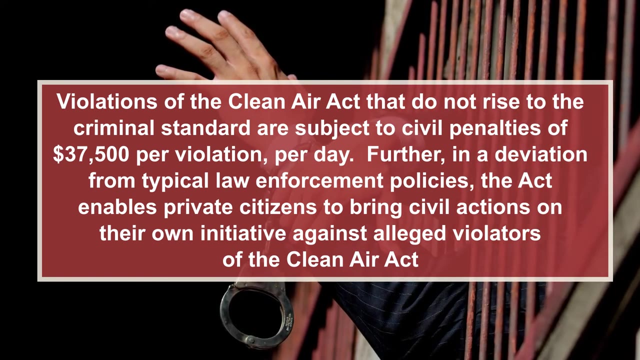 of a Clean Air Act permit or state implementation plan is a federal crime, carrying with it a penalty of hefty fines and up to two years in prison. Violations of the Clean Air Act that do not rise to the criminal standard are subject to civil penalties of $37,500 per violation per day. 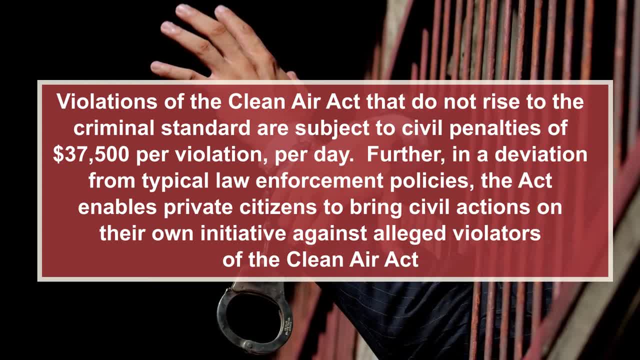 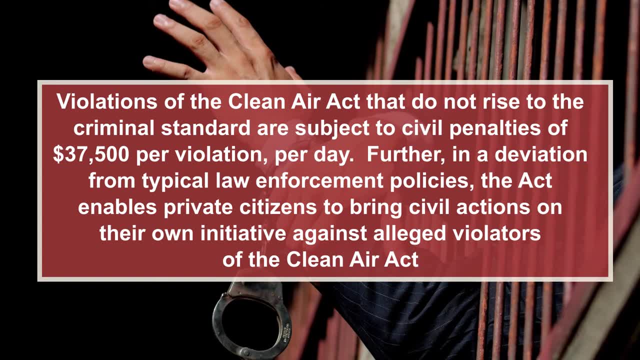 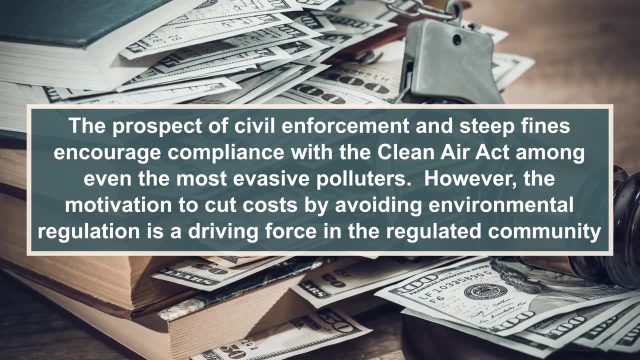 Further, in a deviation from typical law enforcement policies, the Act enables private citizens to bring civil actions on their own initiative against alleged violators of the Clean Air Act. The prospect of civil enforcement and steep fines encourage compliance with the Clean Air Act among even the most evasive polluters. However, the motivation to cut costs by avoiding environmental 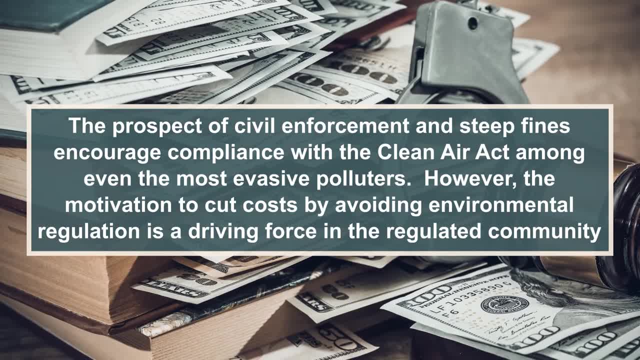 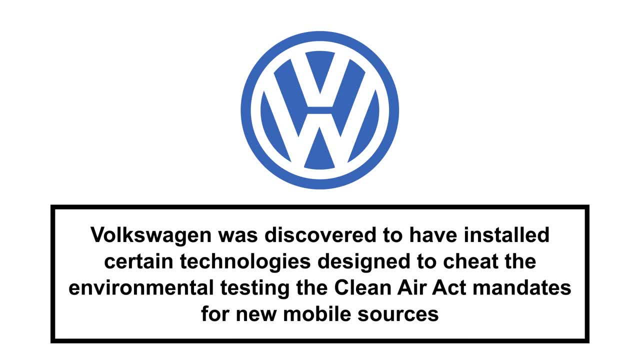 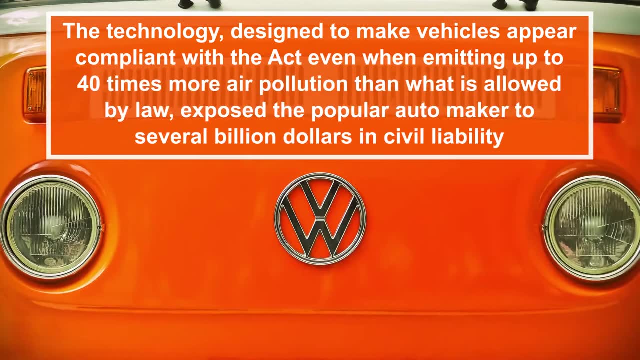 regulation is a driving force in the regulated community. In a recent headline-grabbing scandal, German auto manufacturer Volkswagen was discovered to have installed certain technologies designed to cheat the environmental testing. the Clean Air Act mandates for new mobile sources. The technology designed. 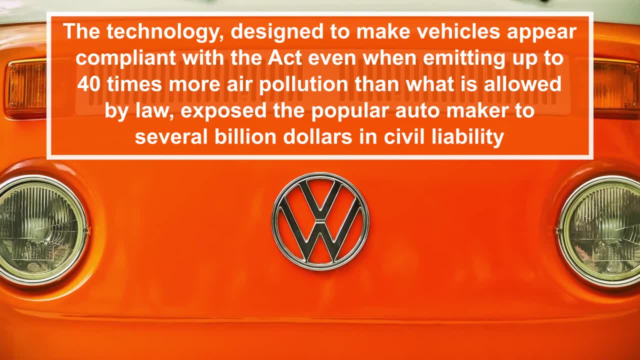 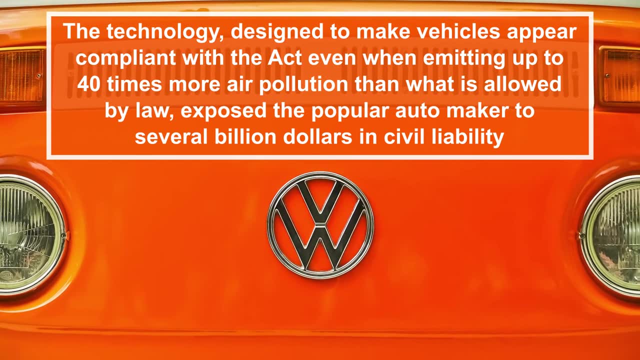 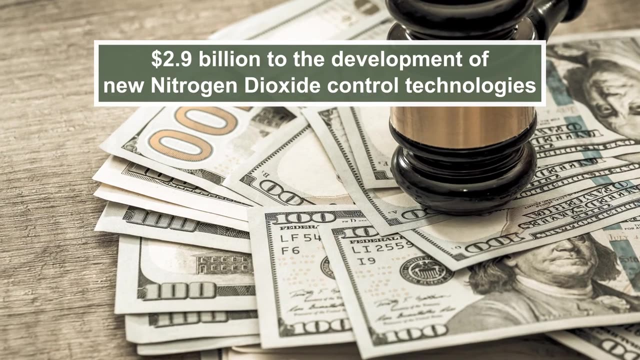 to make vehicles appear compliant with the Act, even when emitting up to 40 times more air pollution than what is allowed by law, exposed the popular automaker to several billion dollars in civil liability. In a settlement reached as part of a plea agreement, Volkswagen committed over $2.9. 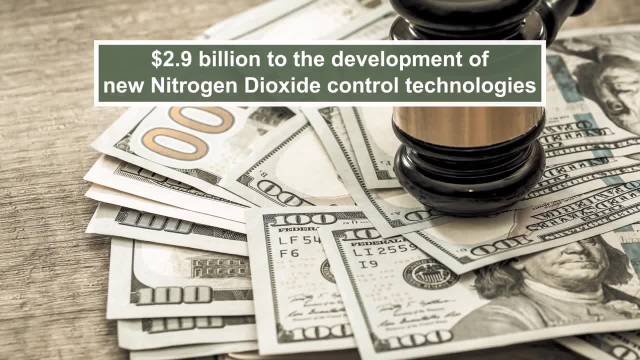 billion to the Clean Air Act. The Act was also used to protect the environment and the environment's quality of life. The company has had more than $10 billion in non-privileged products, including a new new nitrogen dioxide control technology. $4 billion for investment in zero-emission vehicle. 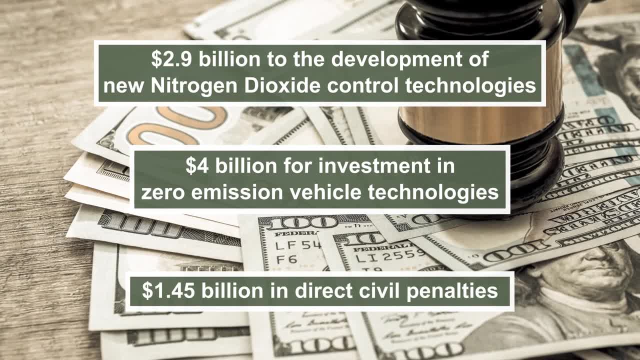 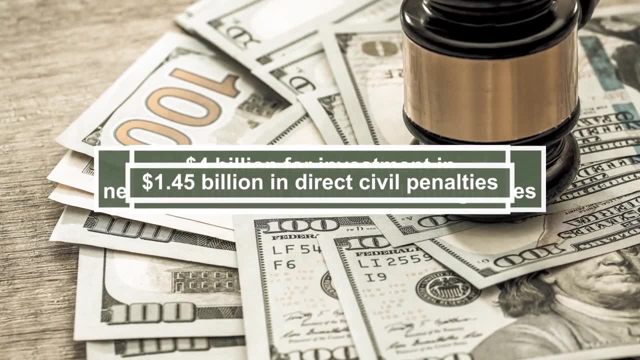 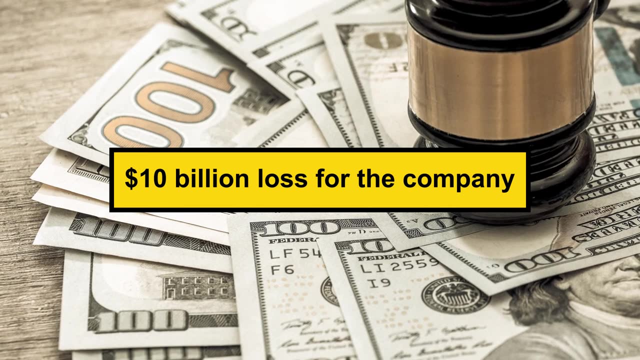 technologies and $1.4 billion in direct civil penalties. These fines, together with other penalties levied against the company for violation of consumer protection laws, are estimated to amount to a staggering $10 billion loss for the company, Although the prospect of being forced to pay 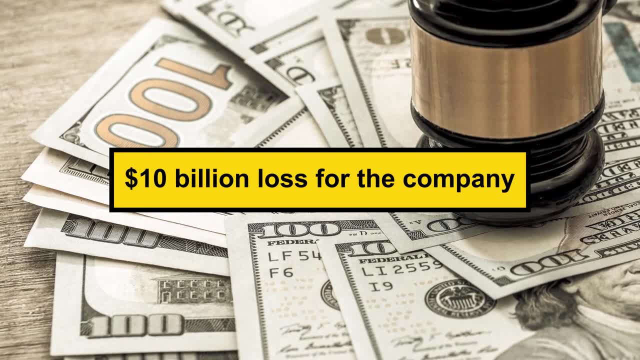 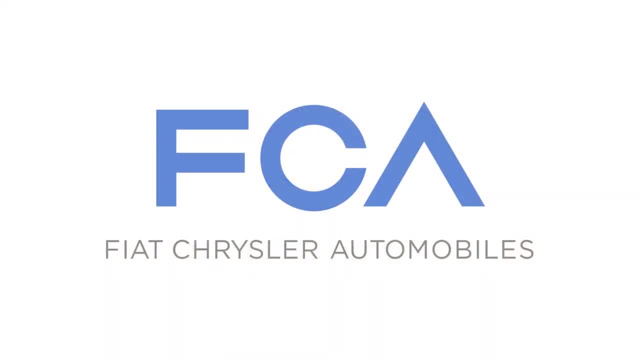 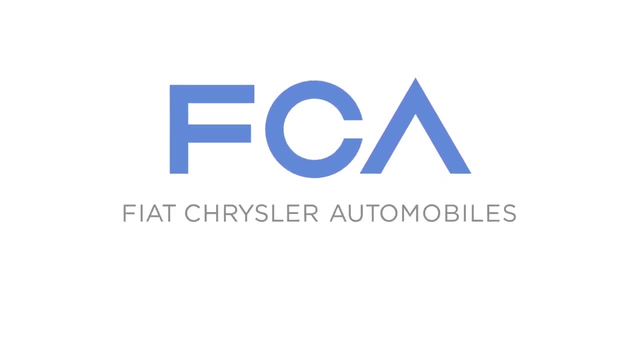 billions of dollars in Clean Air Act fines, penalties and compensation is an obvious deterrent to violations as egregious as intentional cheating. Fiat Chrysler Automobiles is presently facing a civil enforcement action based on facts nearly identical to the Volkswagen emissions scandal. In January 2017, the EPA served Fiat with a notice of violation of the Clean Air Act.